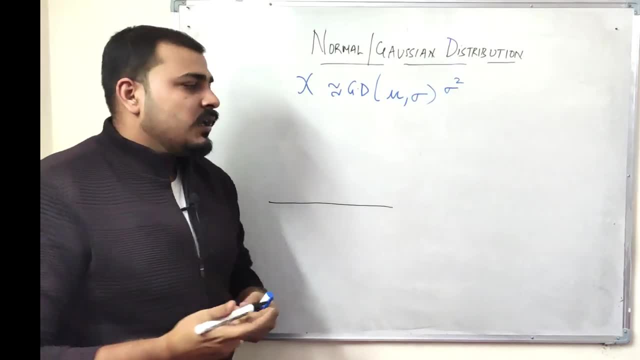 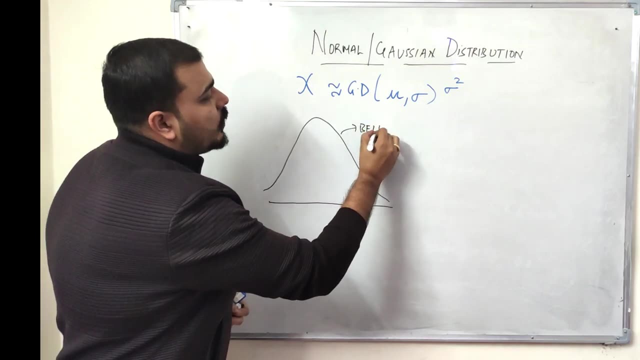 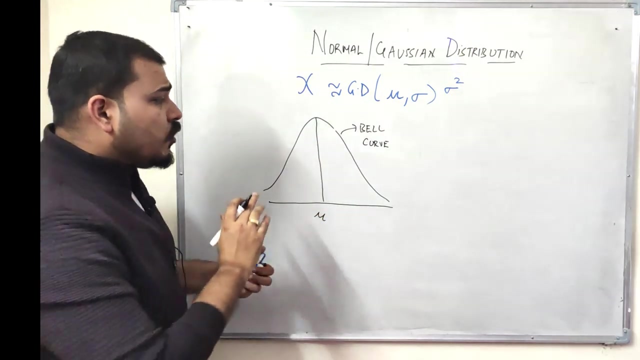 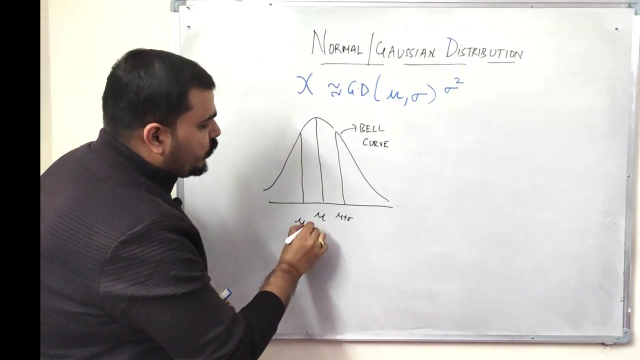 So here let us write y as internal знаю, and this is the random variable, y relatively obvious. This is called constant Goddess function and we use this step in the study of the real world. So let us start off with a very simple step: feeling seminars. 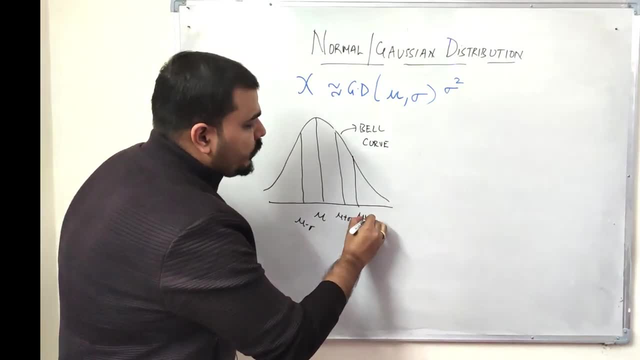 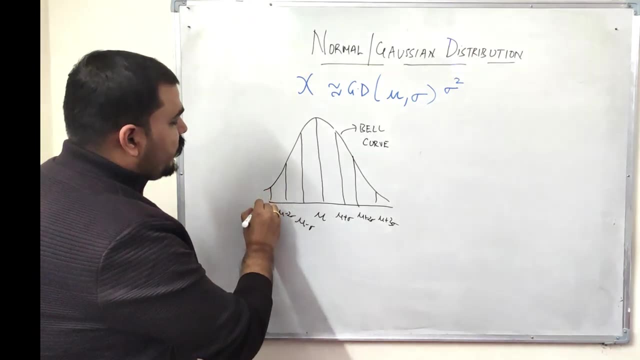 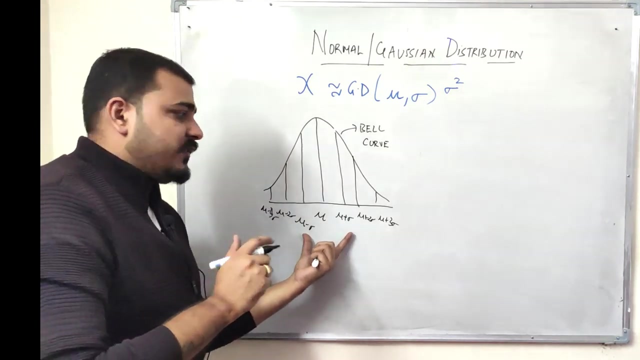 here I will take our transforms two steps first. Now, similarly, your transform, two steps: 2 sigma, this is mu plus 3 sigma. If I go to the left, mu minus 2 sigma and mu minus 3 sigma. Now, this region specifies the range of first standard deviation. So this region 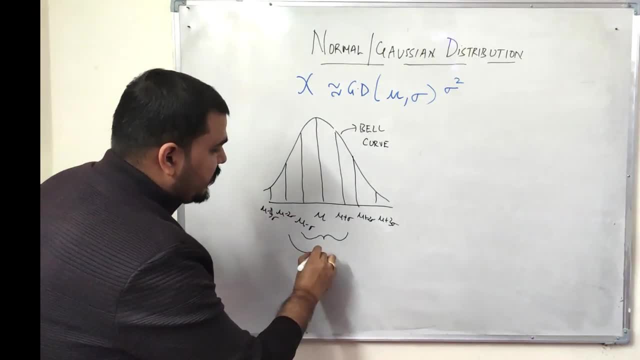 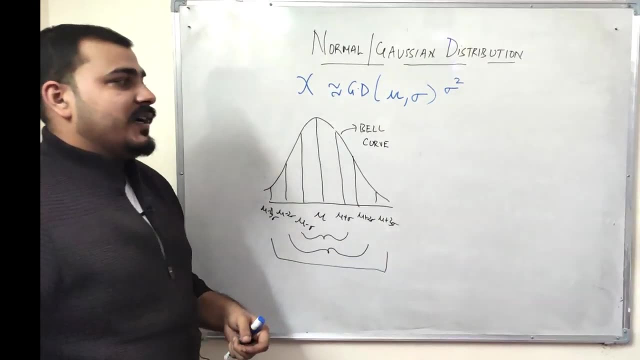 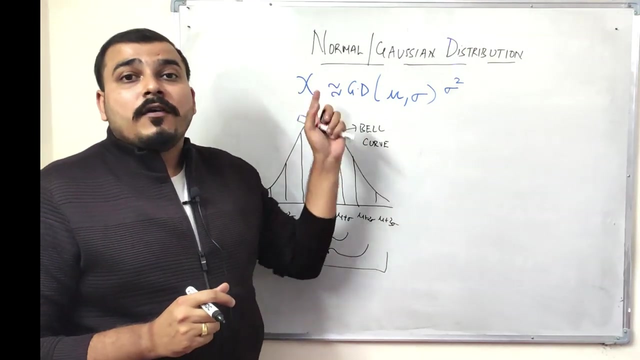 specifies the range of first standard deviation. This region is my second range of standard deviation. I mean range of second standard deviation and similarly for the range of third standard deviation. Now, this bell curve is very, very important thing, and if this random variable follows a Gaussian distribution, it also has three properties. Now that properties? 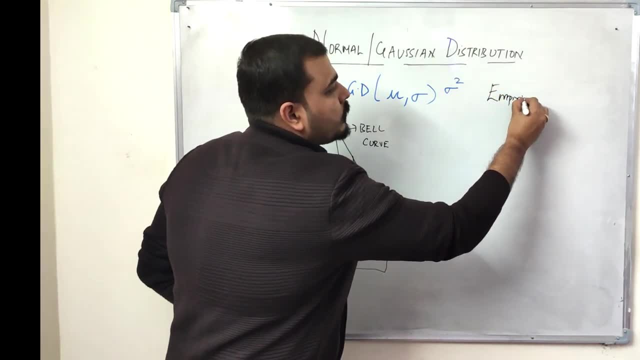 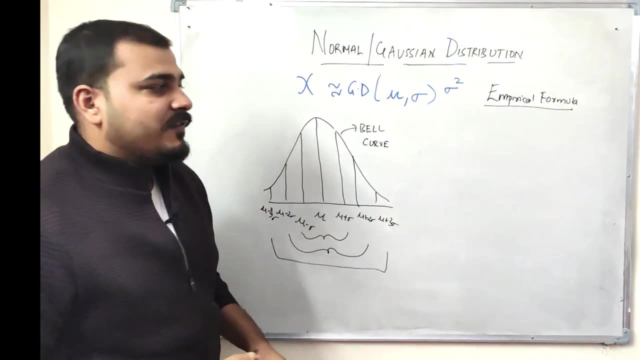 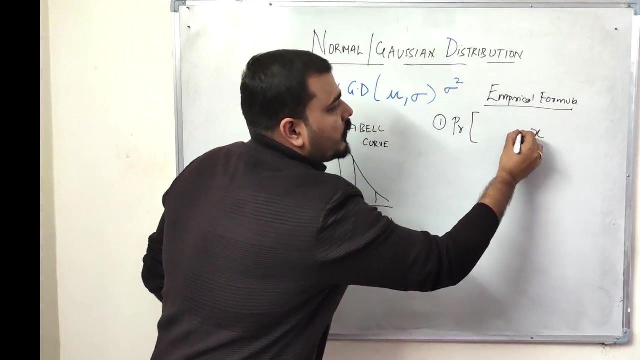 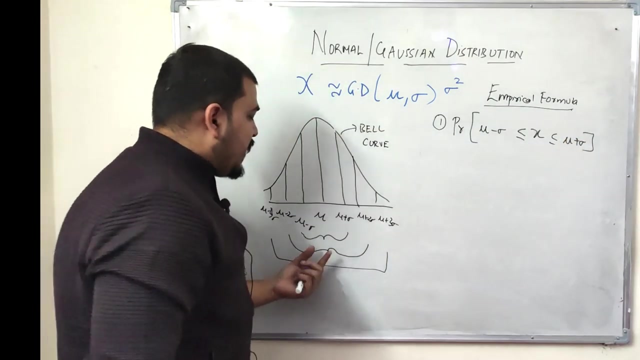 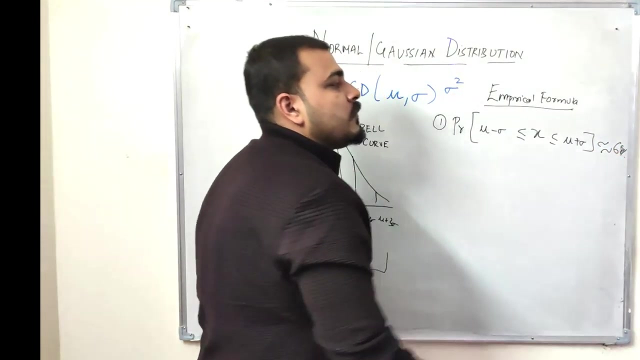 are basically called as empirical formula. Now, what does this empirical formula specify? So first formula basically says that the probability of a variable right that falls within the range of mu minus sigma and mu plus sigma, which is basically my range of first standard deviation, will approximately be equal to 68%. Okay, again, I'm. 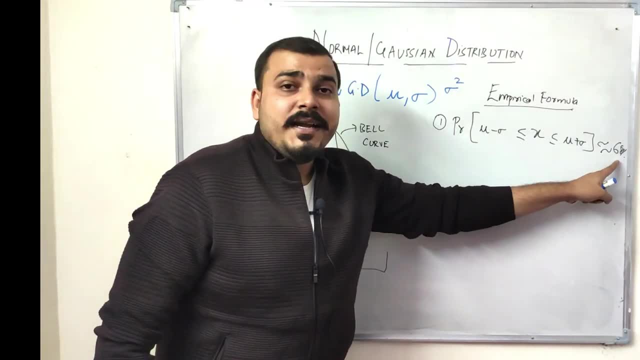 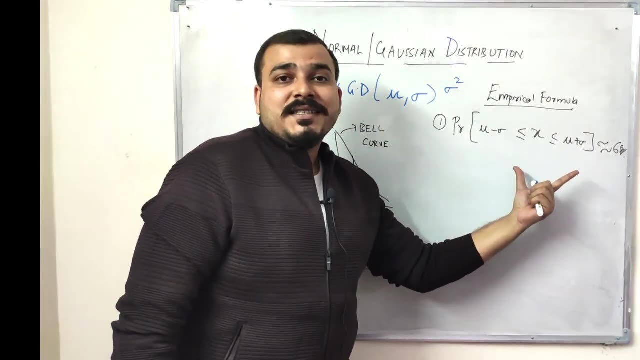 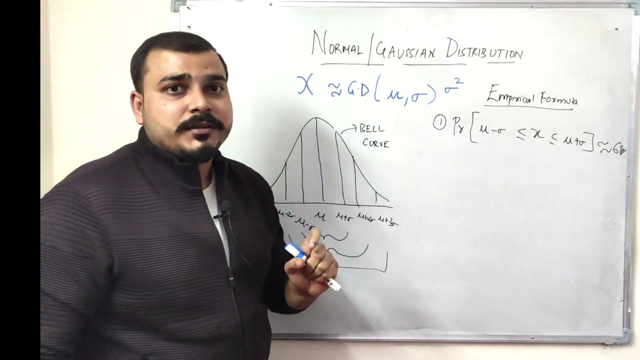 saying that? what does this mean? 68% of the data points belonging to the random variable x fall within the range of first standard deviation. Very much simple. And why? we are saying that? Because this random variable belongs to a Gaussian distribution. Now, similarly, the second point. 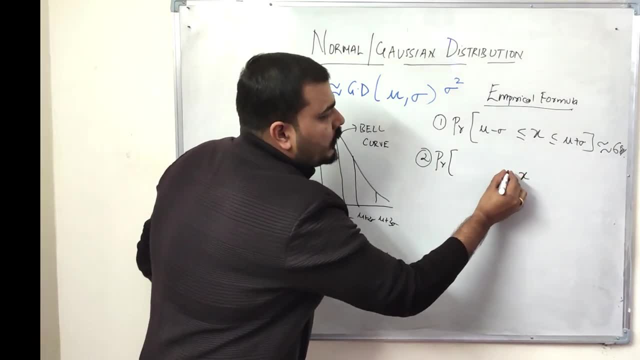 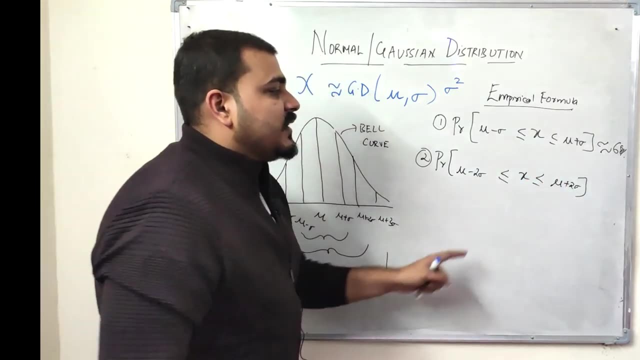 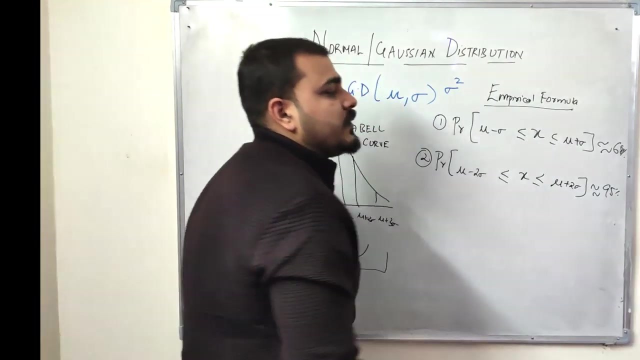 says that the probability of a variable that falls between mu minus 2 sigma and mu plus 2 sigma, when I say this variable, this variable belongs to this random variable. okay, This is approximately somewhere around 95%. This is somewhere approximately around 95%. Now what? 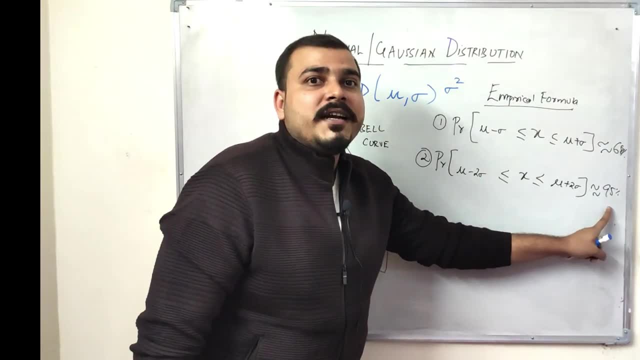 does this specify? This specify 95% of the data points belonging to the random variable x. So this, let's say, think about two gouvernance values- qa of the points belonging to the random variable x and of the data points belonging to this random variable Fall within the range of two standard.